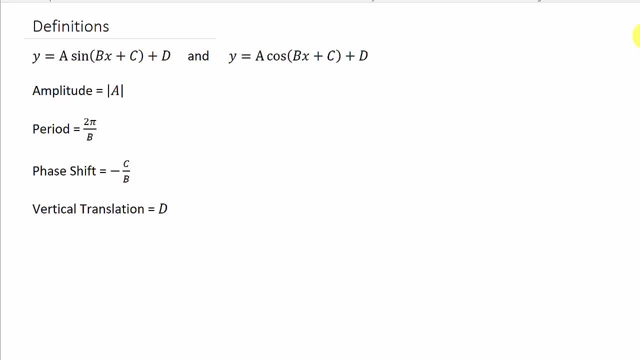 All right. so this video we're going to look at finding amplitude, period, phase shift and any vertical translation. So let's look at it for sine and cosine tangent and all the other ones. they're similar, All right. so here we've got y equals a sine of bx plus c plus d and y equals a cosine bx plus c plus d. And here's your formulas to find the phase shift, the amplitude, the period and the vertical translation. 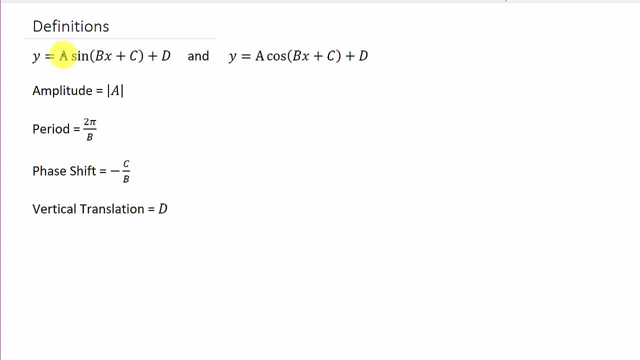 All right, so the amplitude is just the absolute value of whatever's in front of the trig function. Okay, you can see, it's the absolute value of a. a is the part in front of the trig function. The period is 2. pi over b. Okay, b is the number in front of x. here The phase shift is negative: c over b, There's c and there's b. 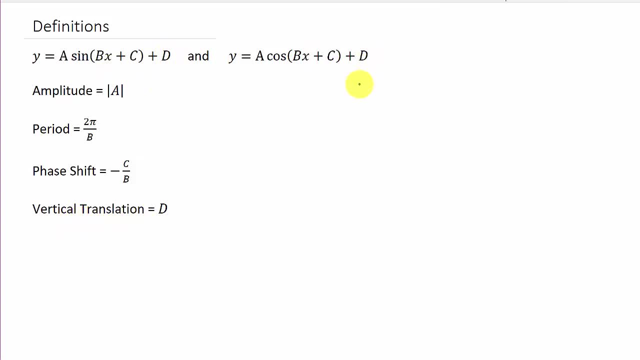 And then the vertical translation is negative: c over b. And then the vertical translation that's d. Okay now the phase shift tells you how the graph moves left and right, and the vertical translation tells you how the graph moves up and down. 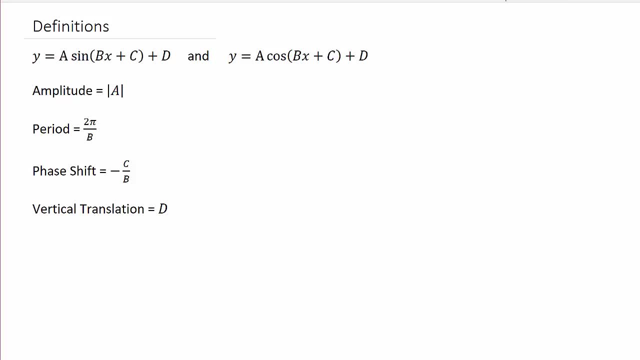 All right, so let's go ahead and get started with the examples. I've got four of them here, And you may want to stay and watch for this one because you see how this one looks different than the other ones. It's got this four and then this: 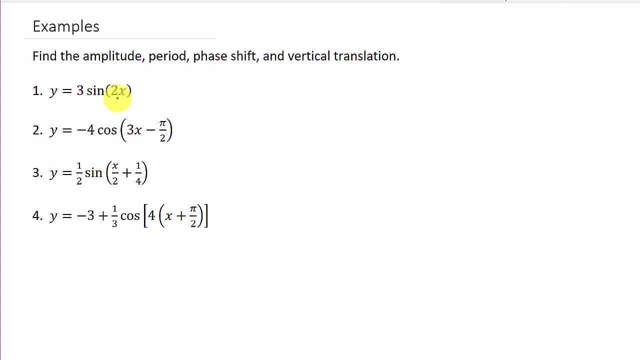 And this is in parentheses, All right. so let's look at number one first. All right. so first, the amplitude is equal to the absolute value of 3, which is just positive 3.. So there's the amplitude. Now let's find the period. 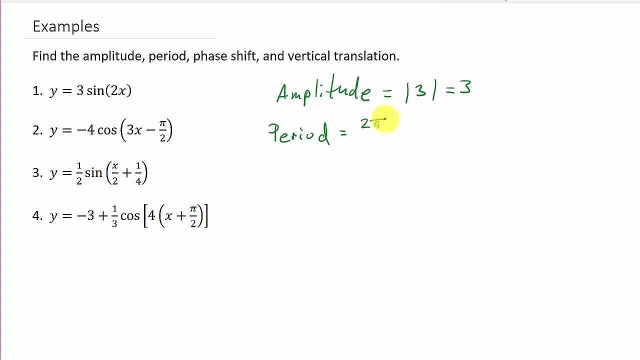 Well remember, the period is 2 pi. It's 2 pi over b. Well, what's b? Well, remember, b is the number in front of x, So b, in this case is 3.. And so there's your period: 2 pi. 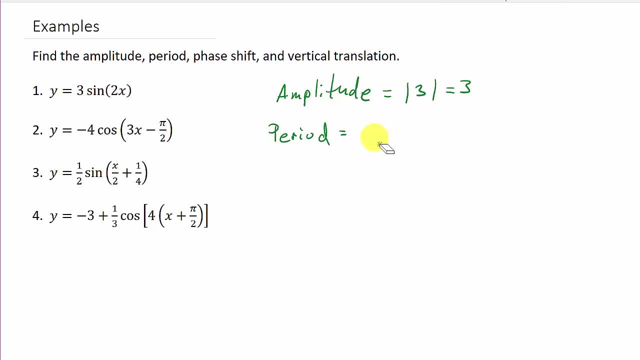 I'm sorry, All right, so now let's find the period. So the period, remember, that is 2 pi over b, And in this case b is 2.. So that's 2 pi over 2, which is pi. 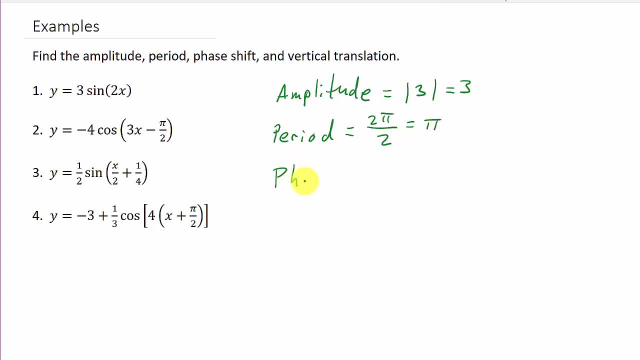 All right, now the phase shift. Okay, so the phase shift is negative: c over b. Well, you can see in this problem, Remember it was bx minus c. Well, all we have is the bx. There's no, I'm sorry, the formula was bx plus c. 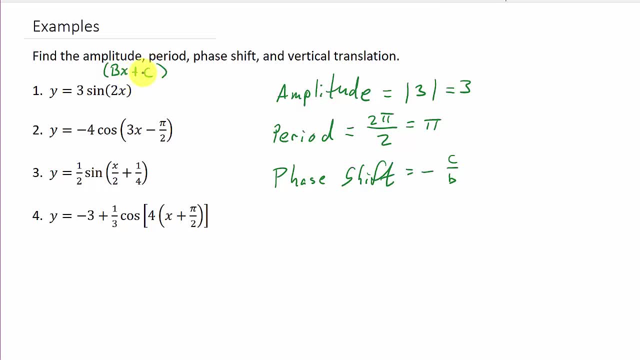 So the formula had this: plus c. Well see, we don't have a plus c here. So in this case c is 0. So our phase shift is just 0. But if you wanted to plug it in, you could plug in 0 for c. 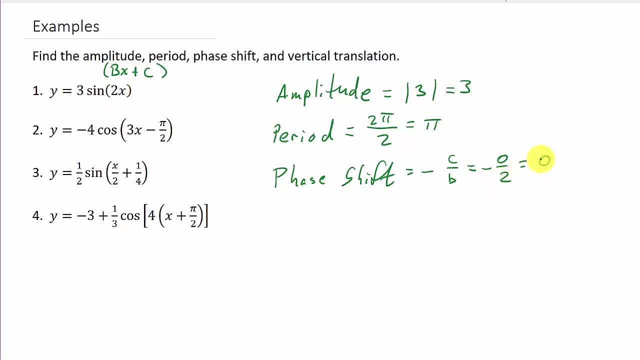 And 2 for b, which would be 0. So there's no phase shift. And then also remember we had that, what the plus d out here? You had sine and the a. Well, there's no plus anything out here. 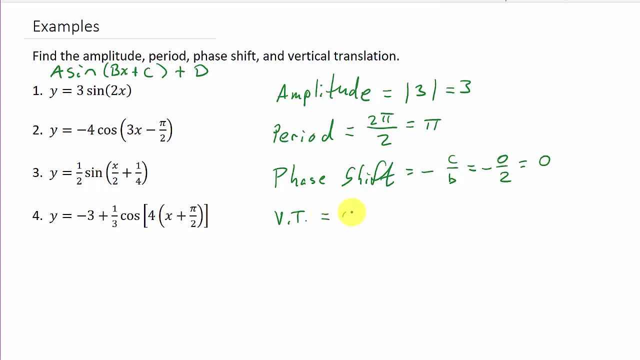 So the vertical translation is 0.. There's none? Okay, All right, so let's look at a Another one, And I'm going to give you a little hint, also on a way to find the phase shift, if you don't remember the formula. 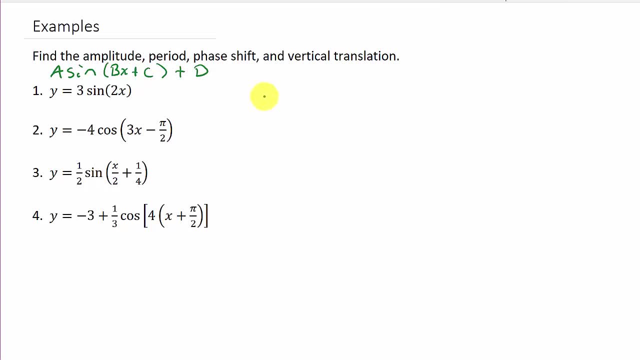 All right, so let's look at number 2.. So number 2, we have the amplitude is the absolute value of a, And we can see a is negative 4.. And so the amplitude would be 4.. The period: The period is 2 pi over b. 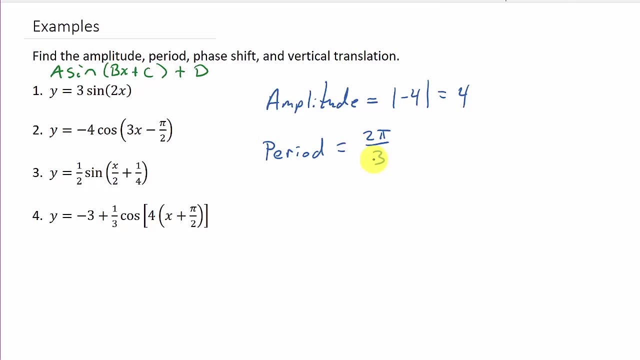 And in this case b is 3.. Okay, Phase shift, All right. so the phase shift, that's negative. c, Okay. So what is c? Well, remember, it's plus c And here we have minus, So c is negative, pi over 2.. 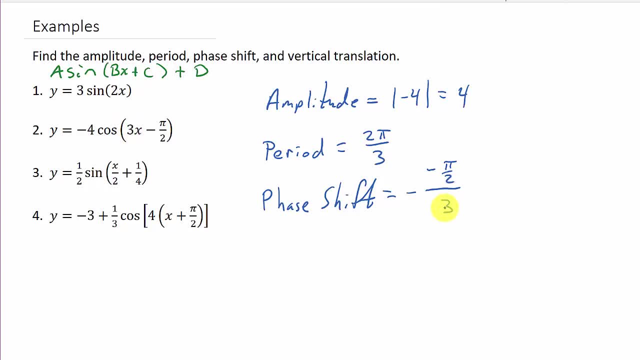 And then b is 3.. All right, So this is going to be pi over 2 over 3.. The negative and negative make a positive, And this is pi over 2 divided by 3.. Or we can look at it as 3 over 1.. 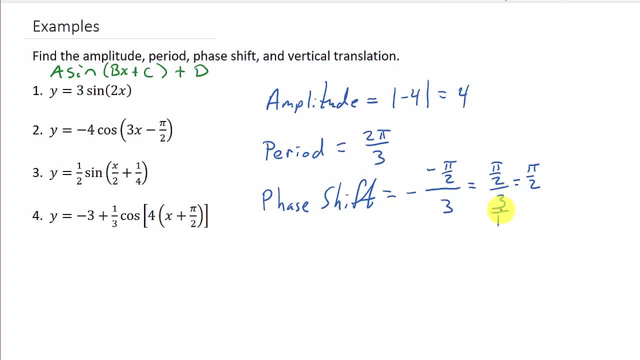 So that's going to be what Pi over 2 divided by 3. Or pi over 2 times the reciprocal, So times 1, 3rd, And so we get pi over 6.. There's your phase shift, And then notice there's no plus d out here. 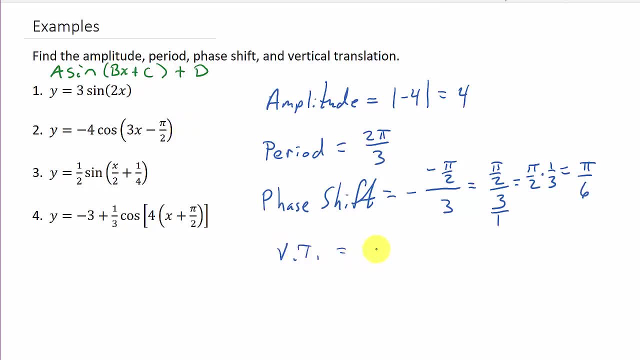 That doesn't have it. So the vertical translation: 0.. There's no vertical translation. Okay, All right, Let's look at the next one. All right, So for number 3,. all right, let's find the amplitude. 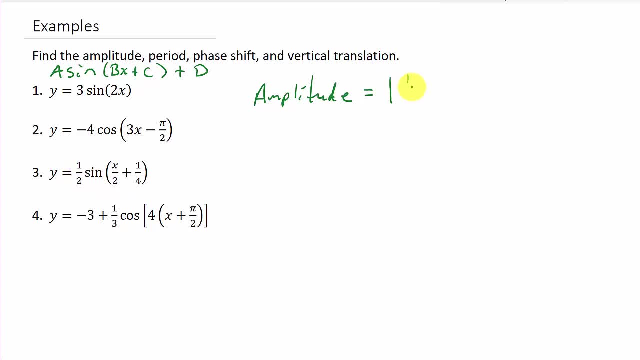 Well, that's the absolute value of a. a is 1 half, So the absolute value of 1 half is just 1 half. The period is 2 pi over b. Okay, Now remember this: x over 2, that is the same thing as 1 half x. 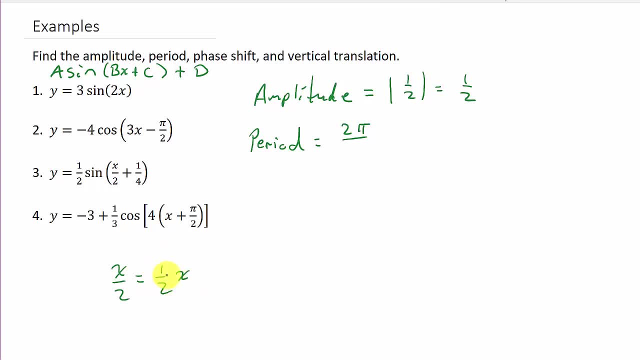 So 1 half is the number in front of x. So 1 half, I'm sorry, 2 pi over 1 half, 2 pi over b, And so that's going to be what: 2 pi divided by 1 half, or 2 pi times the reciprocal. 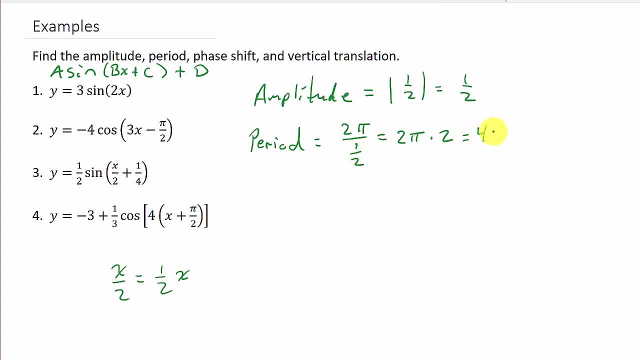 So times the reciprocal of 1, half is 2., And so this is 4 pi. And then the phase shift. that's negative c. Well, in this case c is positive 1 fourth, So that's 1 fourth over b. 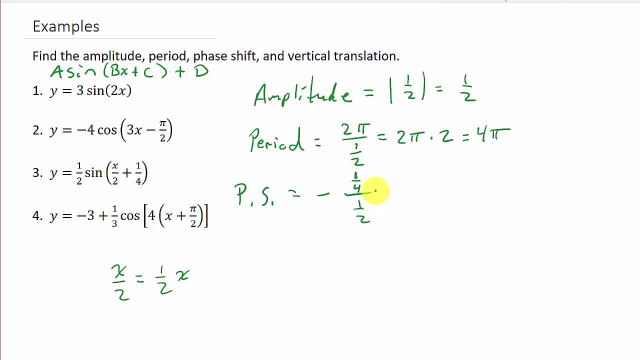 And remember we saw that b was 1 half. Okay, So that's negative 1. fourth times the reciprocal of this, So times 2 over 1.. And so that's That's negative 1 half. And then the vertical translation. you can see there's no plus d or anything. 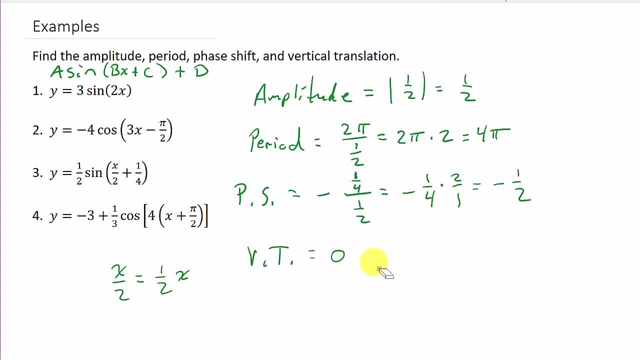 So that is just 0.. There's no vertical translation, All right. So what I want to mention to you before I start, the last problem is the phase shift, that minus c over b. Look to find the phase shift. all you have to do. you see what you're taking the sine of. 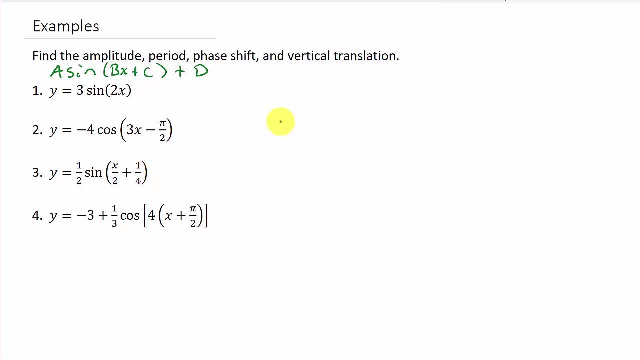 or what you're taking the sine of? you're taking the sine of. you're taking the sine of, or what you're taking the cosine of? okay, Whatever that is. all you have to do is take that, set it equal to 0, and solve. 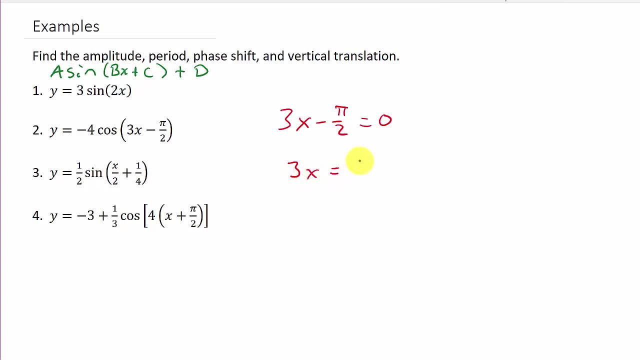 So if we move the pi over 2 over, we get 3x equals pi over 2. And then we multiply everything by 1 third to get rid of the 3. So x equal pi over 6.. That's another way you can do the phase shift. 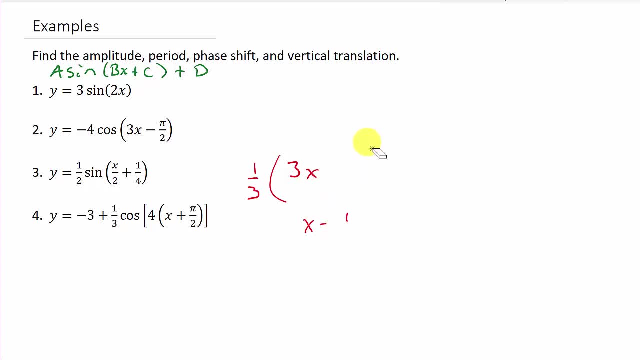 Just whatever you're taking, And the sine or cosine of just set it equal to 0 and solve for x. All right, All right. So now let's look at the last problem. Now, if you notice, this one's in a little bit different format than the other ones. 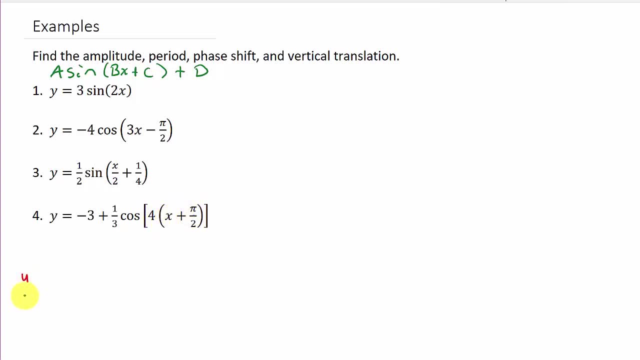 Okay, This part here is different. So what this is is. this is in the form a cosine: bx plus C plus d. Now, I know the d is over here and not back here behind the. that's, that's fine. 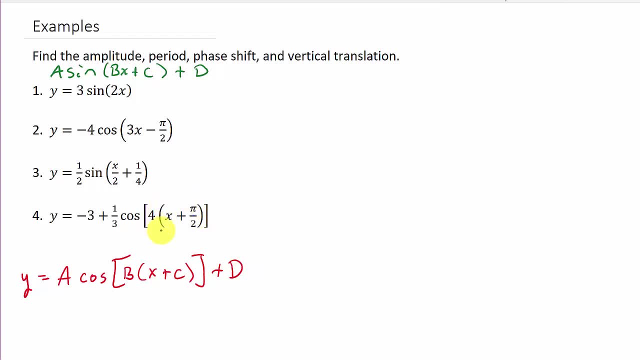 Okay, That's not a big deal. What we're looking at is this right here. Okay, So let's just go ahead real quick and get the, the amplitude and the period, and then we'll talk about the phase shift, Okay. 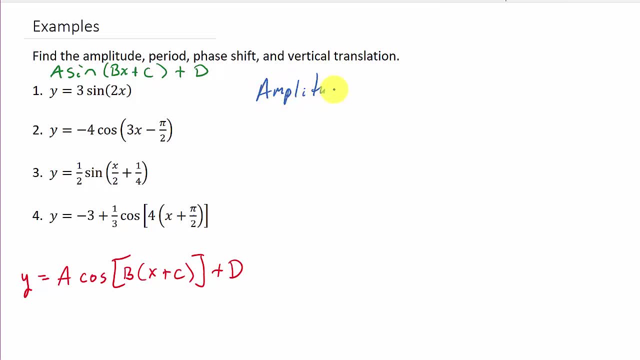 So the amplitude Is just the absolute value of a, and in this case a- that's the number right in front of cosine- is one-third. So that's the absolute value of one-third, which is just one-third. And then the period. 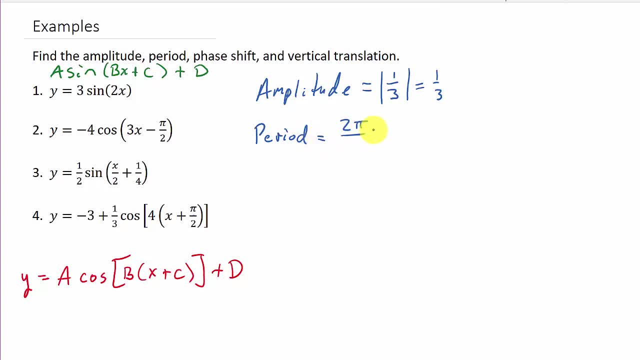 Okay, So the period, remember that is 2 pi over b. Well, what's b? Well, you can see, this is b, the number right in front of the parentheses. So that's 4.. b is 4.. 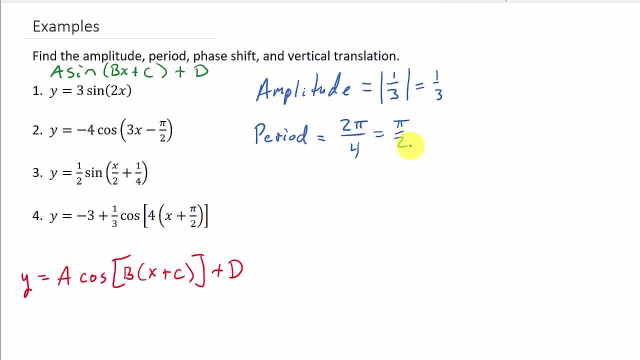 And so the period is pi over 2.. Okay, Now let's look at the phase shift. Now I'm going to find this two different ways, but I'm going to show you. I'm going to show you how, how this works out. 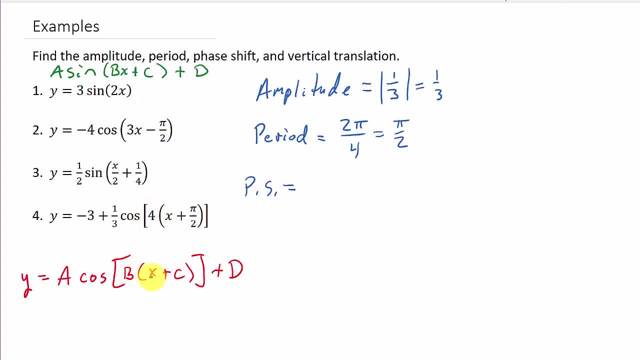 All right. So with the 4 out here, see how. how this b is outside the parentheses. See, everywhere else is just right up against the x, except for here. It's separated from the x and the Pi over 2.. 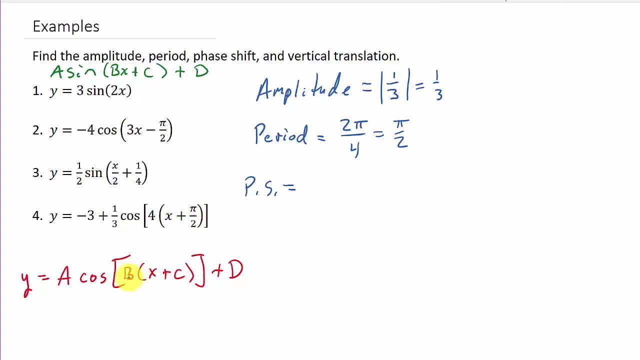 All right. So when this happens, your phase shift is just negative c, So this would be negative pi over 2.. And that's your phase shift. Okay, Now let me show you how that works out. So, if this, if you distribute this, okay, if you distribute. 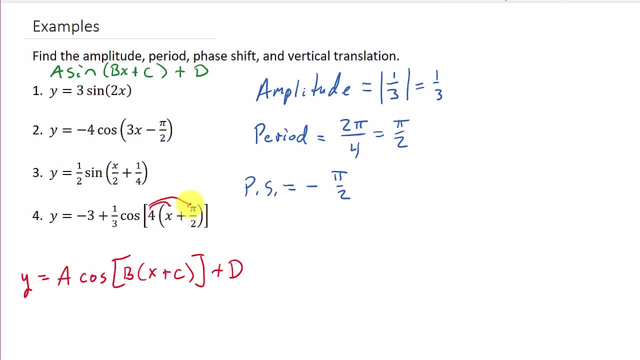 Then you've got cosine 4x plus 2 pi, if I distribute the 4.. Okay, So now let's go ahead and find the phase shift, like we did in all of these. It's what Negative c, And I'm using this one now. 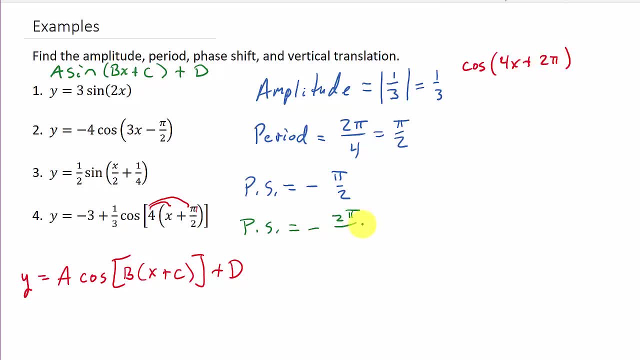 Negative c, c is 2.. 2 pi Over b, And what's b, b is 4.. And so that's, And so that's negative pi over 2.. Now let me say this: Some books will put the problems like this: